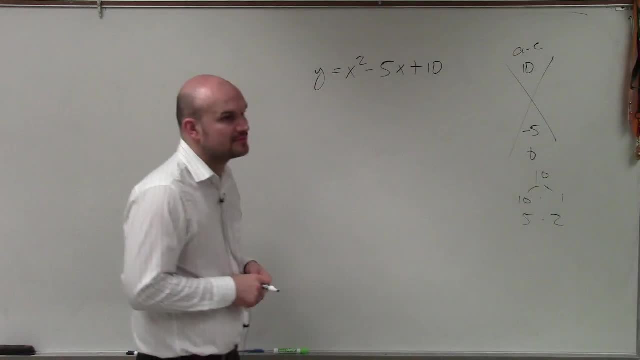 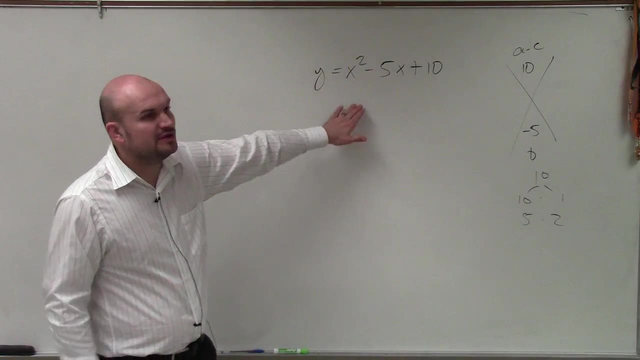 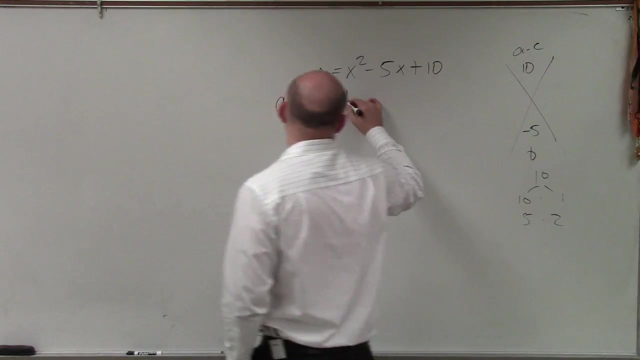 though, is to be able to use the quadratic formula to be able to solve the values for x. So what we're going to do for that is first a couple steps. First step is we need to identify a, b and c, and when you guys are doing your work, I want you to do it just like I'm doing. 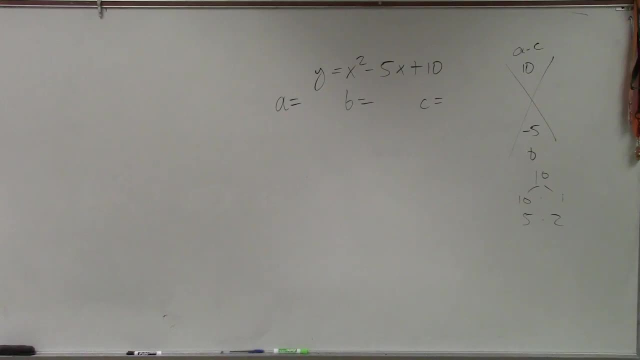 right up here. I want you to say: a equals this, b equals that and c equals this. Okay, so you're going to write out a, b and c and then you're going to plug in what those values are: 1,, negative, 5, and 10.. 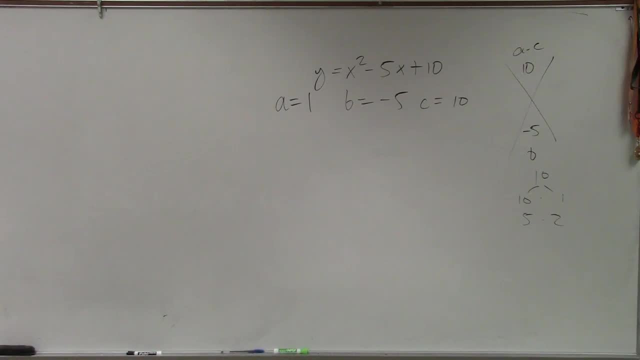 Okay, now, once you go ahead and label this, the next thing to set step number one. Now, step number two is to identify the discriminant. Now, I'm not going to get into much detail on this video for discriminant. Yes, yes, Okay, Jennifer, the homework is on the. 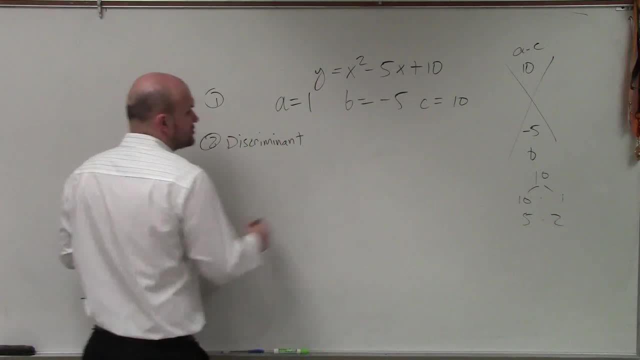 thing. Thank you, Yep, thank you. Discriminant is going to be b squared minus 4 times a times c. So basically, all I'd like you guys to do is just practice finding, determining what the value is of the discriminant. I'm going to explain what exactly I'm the discriminant- a little bit more, not in. 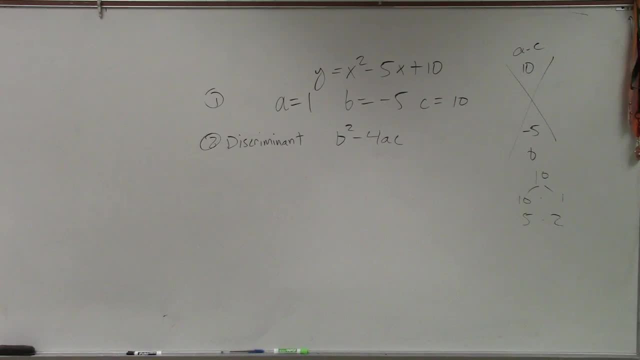 this video, though, but I will explain it. So I'll explain it in a little bit more detail to you next time, but for right now I don't. we haven't gone into it, and I will go over it. 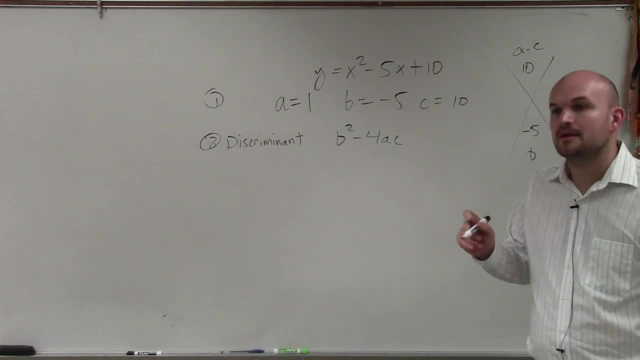 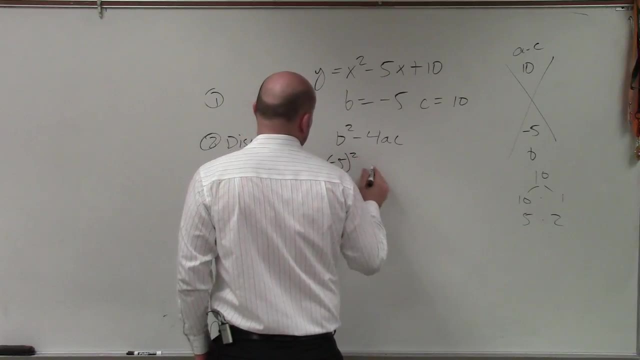 If you solve it in quadratic formula, what is the formula? We're going to get to that. We're going to get to that Right now. I just want you to identify the discriminant which is negative: 5 squared minus 4 times a, which is 1, times c, which is 10.. 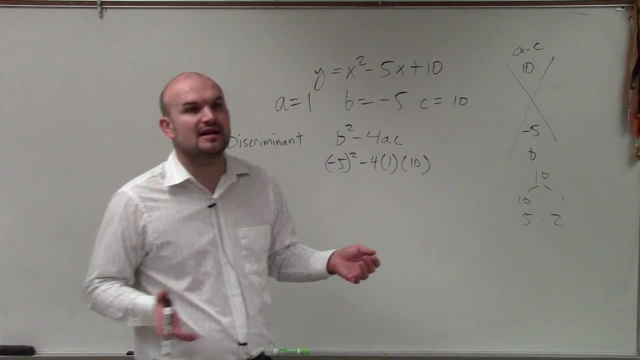 So does everybody see what I did? I just took the values for a, b and c. It's out of the printer in the printer box, So I just took the values of a, b and c and I plugged them into this. 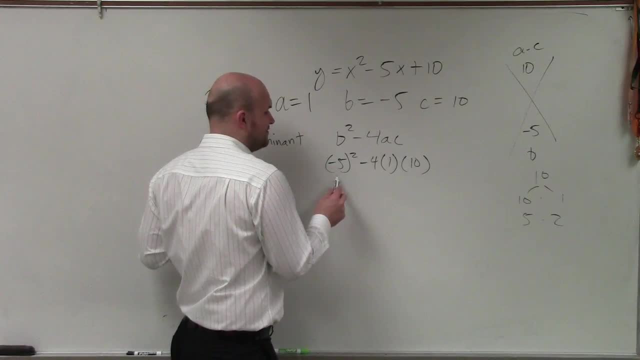 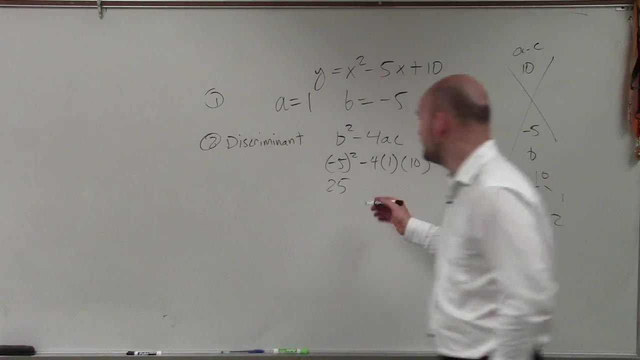 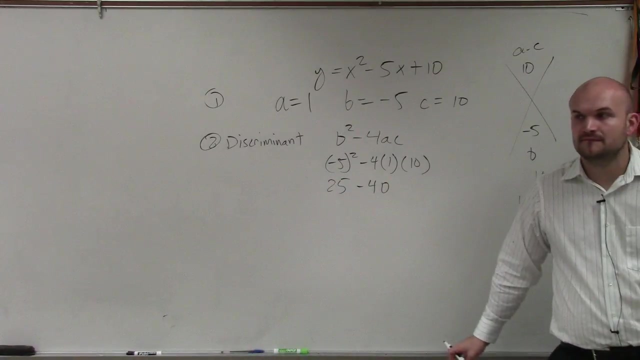 little formula Now. I basically remember: negative 5 squared is positive 25.. And then negative 4 times 1 times 10 is going to be a negative 40. Correct, Yeah, Everybody understand, Agree with me. Then I just do 25 minus 40 and I get negative 15.. 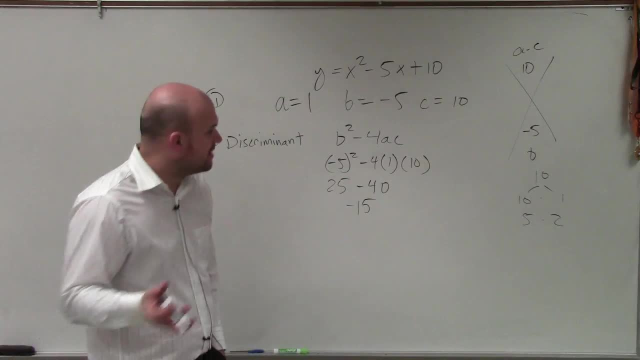 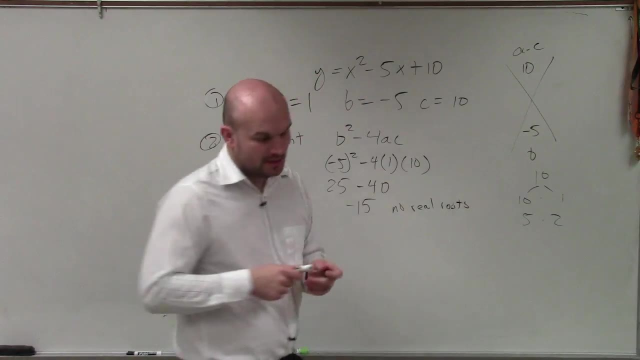 All right. Now again, as I mentioned, when we go over this, whenever you have a negative, I just want you guys to write in: no real roots. You're not going to have real roots, You're going to have complex roots for this example. 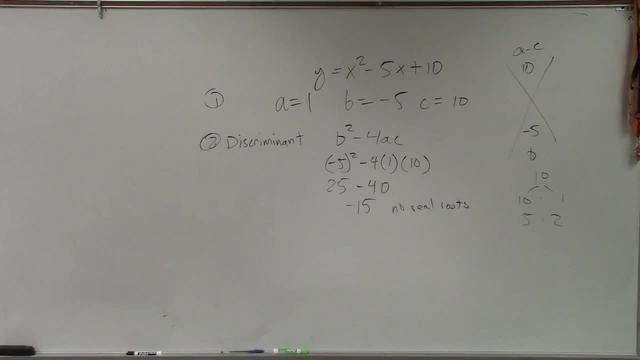 But I'm not going to get that in depth with all of this. We're basically just going to go over what you guys need to remember from your Algebra 2.. All right, Brittany, Then you would have gone over this, which would have been nice. 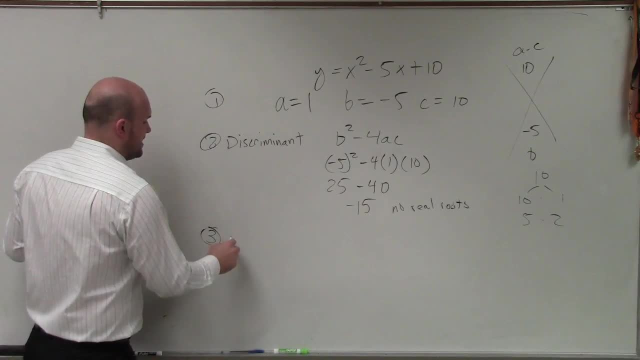 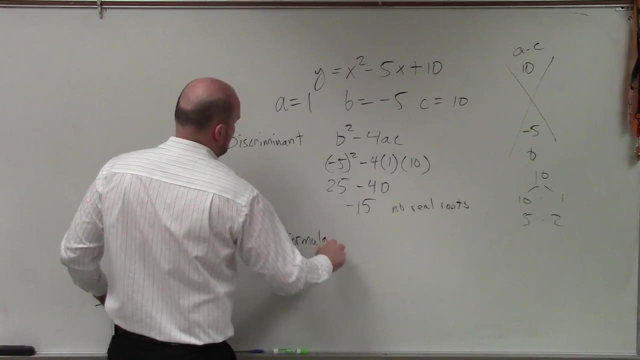 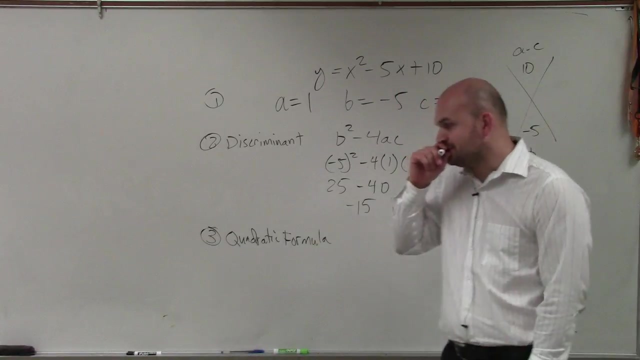 Yeah, we've already covered this in Algebra 2.. So then, step number three is applying the quadratic formula, which is actually the formula that we're going to be using. So to use the quadratic formula. remember you guys at the end, when we were solving these. 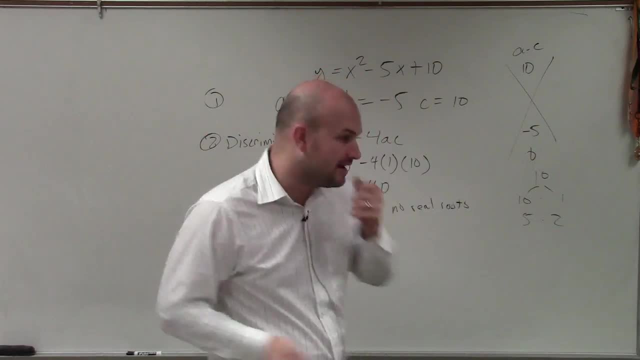 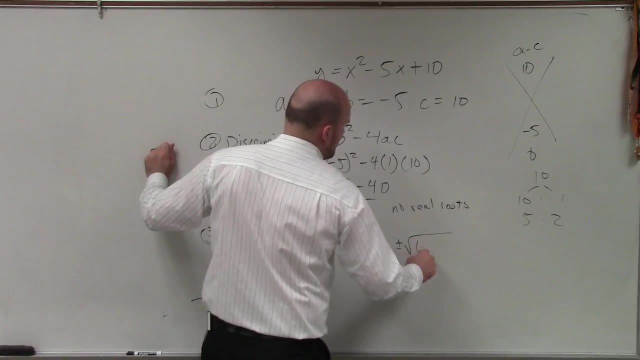 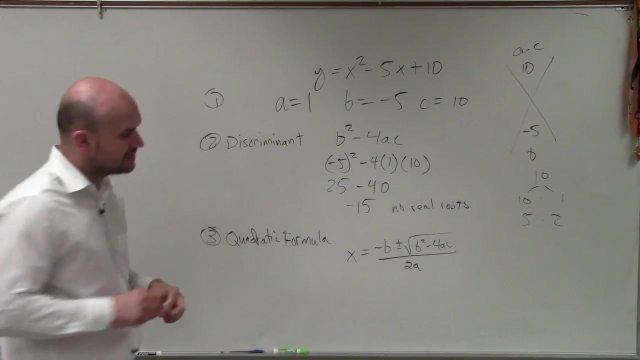 we got x equals right. When we factor at the end, x equals our values. So the quadratic formula is the solutions for x And the formula goes opposite of b plus or minus b squared Minus 4 times a times c, all over 2a. 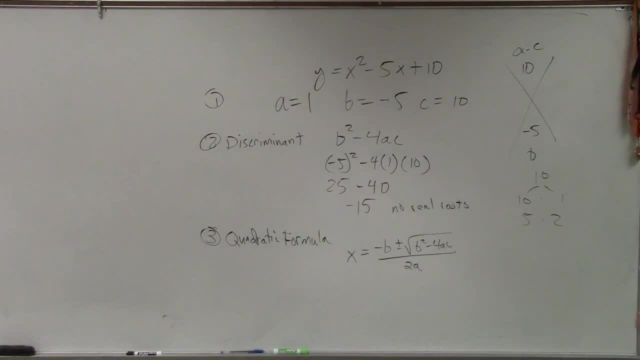 Now a couple things that I want you guys to understand about this quadratic formula is: the discriminant is what is under the square root. So we already solved part of this problem when we found out what the discriminant was. So, rather than just taking the whole formula, 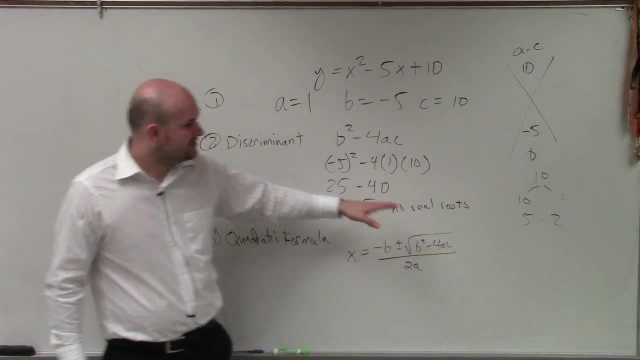 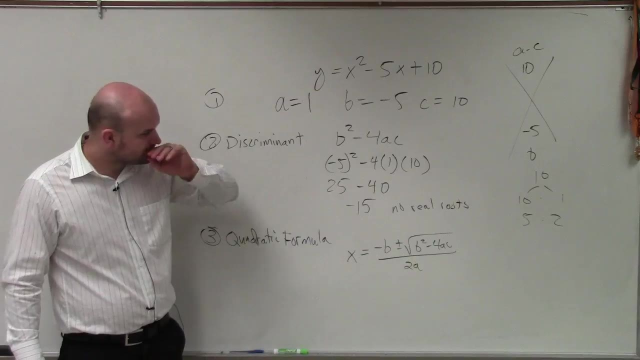 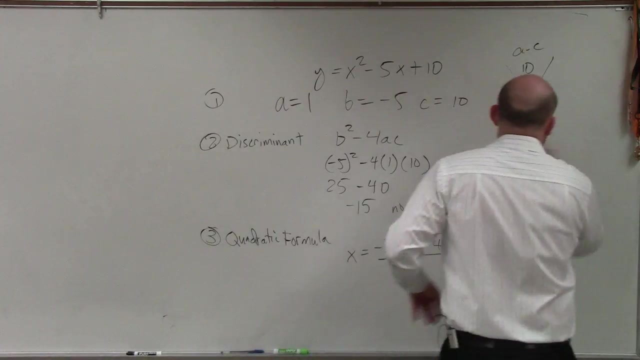 and just plugging in numbers. we went ahead and determined the discriminant, And I'll explain why. we're going to do that again, as I mentioned in another video. So we now have our discriminant. So now to figure out the values. all I'm simply going to do. 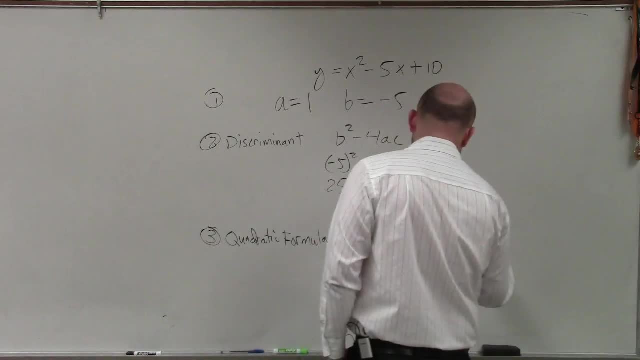 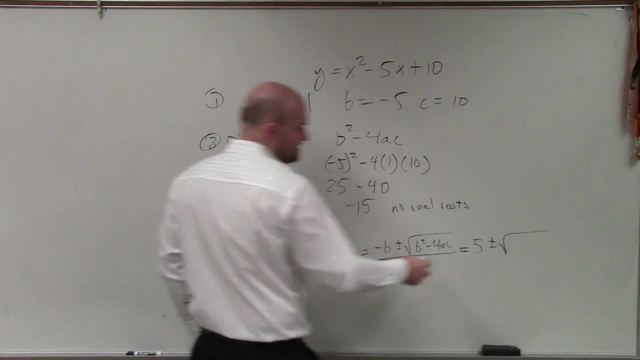 is plug in the values for a, b and c. So I have x equals opposite of b. Well, b is negative 5, so now it's 5 plus or minus the square root of negative 15.. I already found that value. 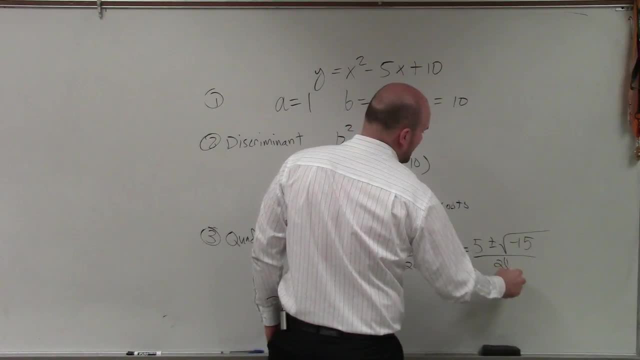 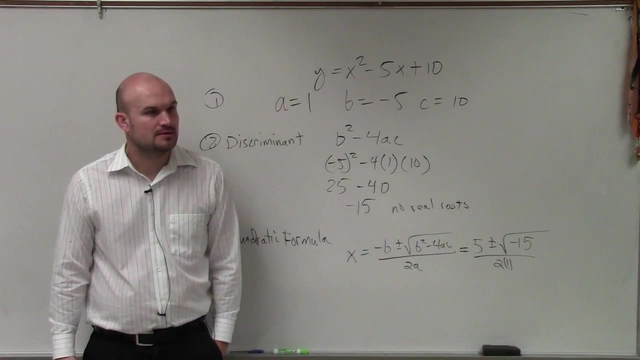 Divided by 2 times a, which is 2 times 1.. So does everybody see what I did there? Yes, no, maybe. so OK, Now, another thing to get with you guys is: we talked about there's no real roots.